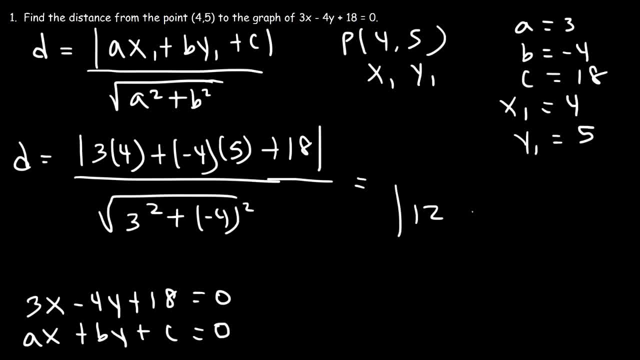 So we have 3 times 4, which is 12.. Negative 4 times 5 is negative 20.. And then 3 squared is 9.. Negative 4 squared is 16.. Now let's make some space. 12 minus 20 is negative 8.. 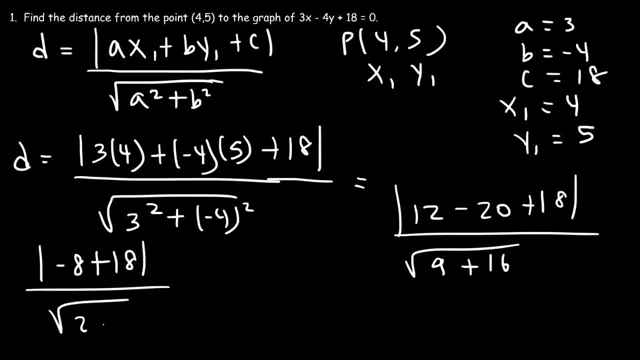 and 9 plus 16 is 25.. Negative: 8 plus 18 is 10 and the square root of 25 is 5.. So 10 divided by 5 is 2.. So that's the distance between the point and the line Number two. find the distance from the. 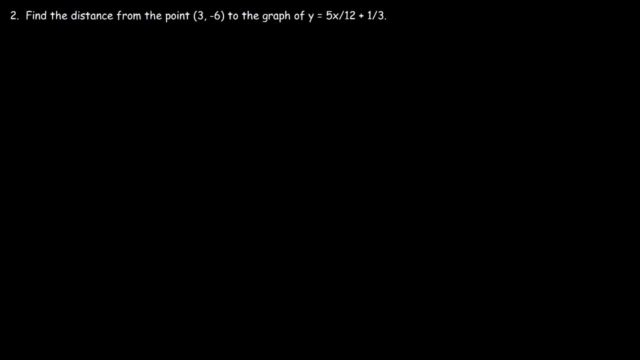 point 3: negative 6 to the graph. y equals 5x over 12 plus 1 over 3.. So we can see that this is x1 and this is y1.. So x1 is equal to 3 and y1 is negative 6.. Now what we need to do is write the. 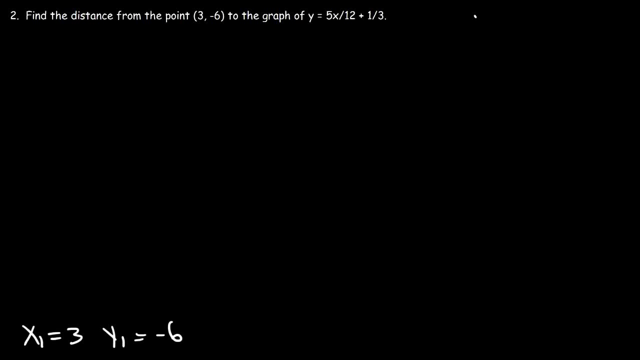 linear equation in standard form, And so we need it in ax plus by plus c equals 0 format. So let's rearrange that equation. So first I'm just going to rewrite it. This is what we have. So I'm going to take everything and 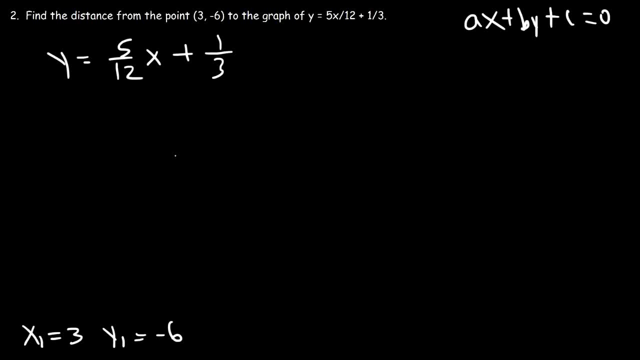 move it to the left side. So what we now have is negative. 5 over 12x, plus y, minus 1 over 3 equals 0.. Now I need to get rid of the fractions, So I'm going to multiply everything by 12.. So negative. 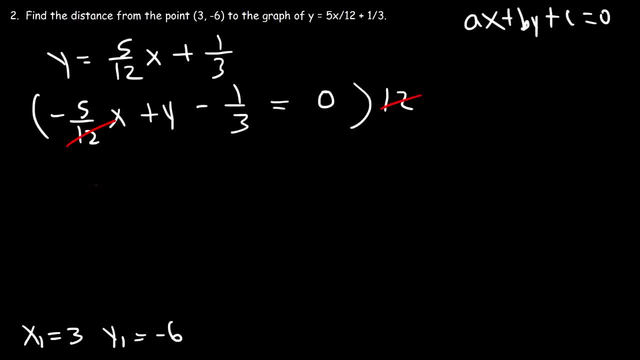 5 over 12 times 12.. The 12s will cancel, giving me negative 5, or rather negative 5x, And then I have y times 12.. So that's going to be positive 12y And then negative 1, third times 12, which is: 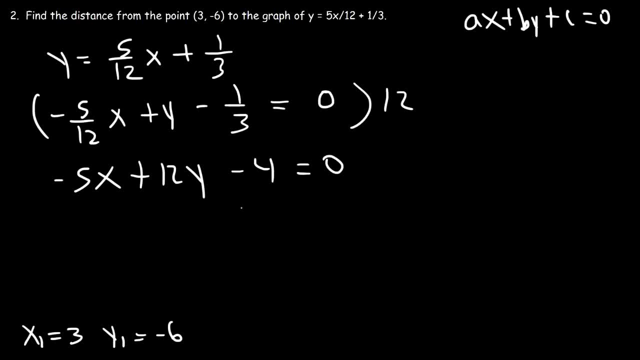 negative 4.. Now if we multiply everything by negative 1, we can say: this is 5x minus 12y plus 4 is equal to 0. So now it's an ax plus by plus c format. So we can say that a is 5, b is negative 12, and c, that's equal to positive 4.. 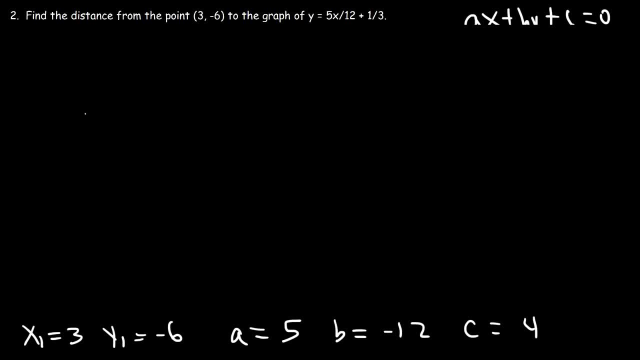 So, now that we have everything that we need, let's start with the distance formula. So d is equal to the absolute value of ax1 plus by1 plus c Divided by the square root of a squared plus b squared. So a in this example is: 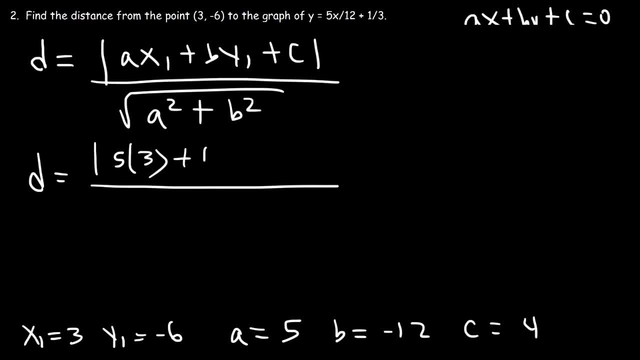 5, x1 is 3.. b is negative 12,, y1 is negative 6, and c is equal to 4.. Now, a squared, that's going to be 3 squared, and b squared is going to be actually a is not 3, a is 5.. Let's fix that. So this is 5 squared. 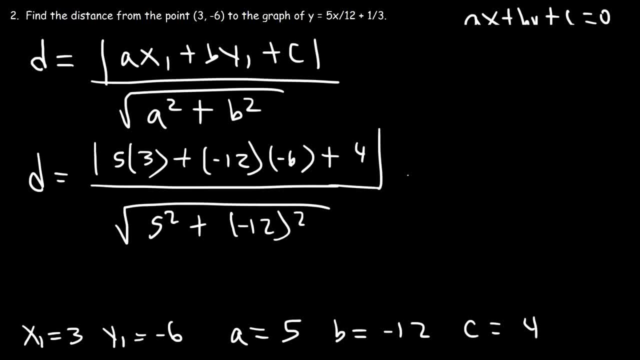 And then b is negative 12.. So now let's do some math: 5 times 3 is 15.. Negative 12 times negative 6, that's positive 72.. Now 5 squared is 25.. Negative 12 times. 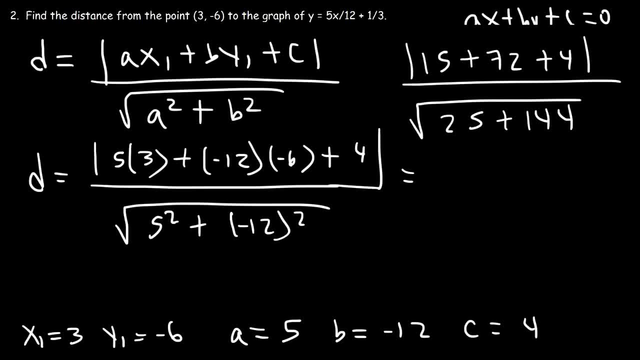 negative 12,, that's positive 144.. Now, 15 plus 72,, that's 87.. And 87 plus 4 is 91.. 25 plus 144 is 169, and the square root of 169 is 13,, and 91 divided by 13 is 6.. 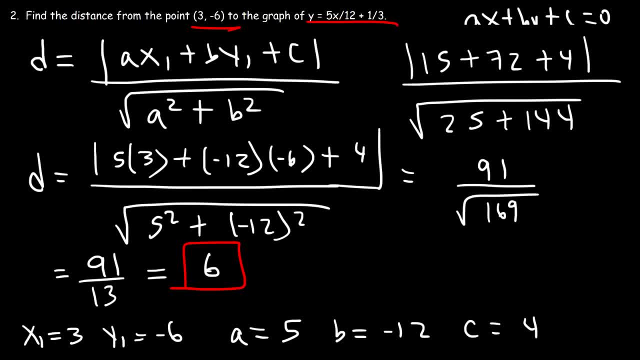 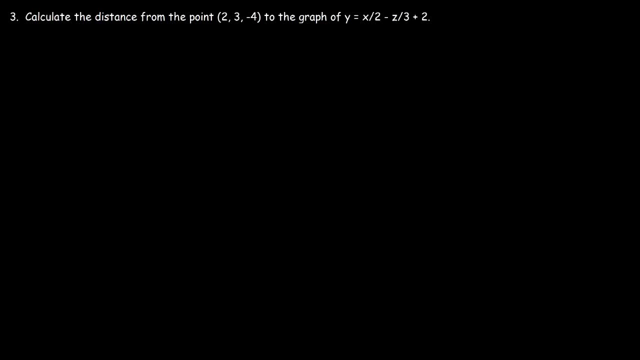 So the distance between this point and this line, that is, the perpendicular distance, is 6 units. So now you know how to calculate the distance between a point and a line in two dimensions. Number three, calculate the distance from the point to the graph of y, is equal. 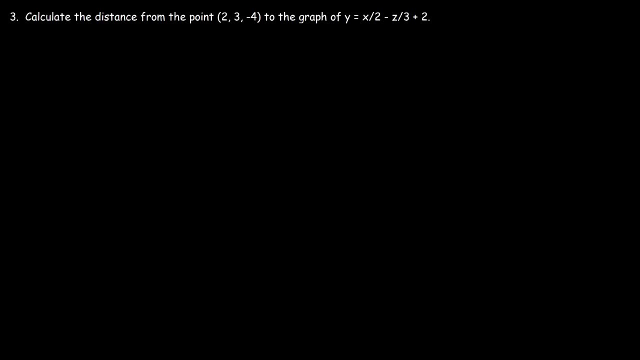 to half of x, negative 1 third z plus 2.. So this is x1,, y1, and z1.. So we can say that x1 is equal to 2, y1 is equal to 3, and z1 is equal to negative 4.. 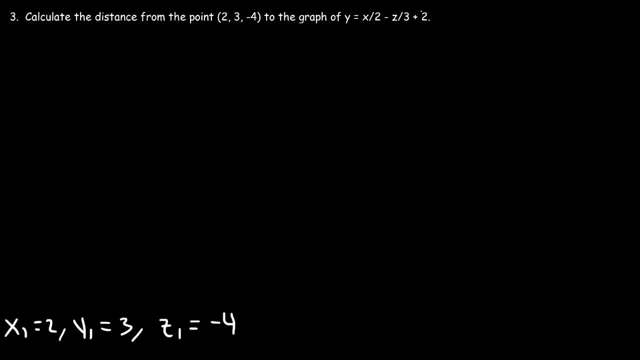 So we have three dimensions in this particular problem. Now let's rearrange this equation. We want to get it in this form, That is, ax1 plus by1 plus cz1 plus d is equal to 0. So let's take everything from the right side and move to the left. 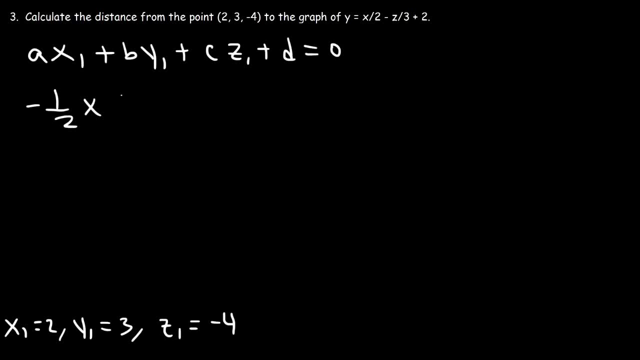 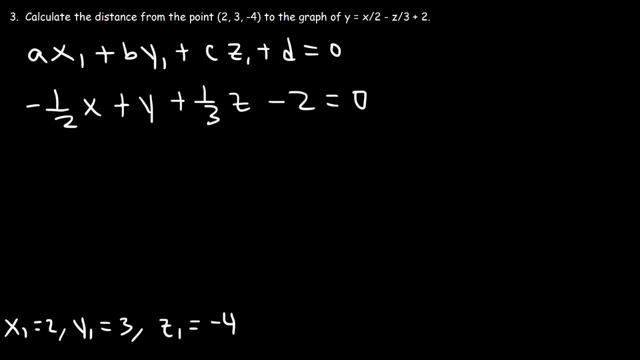 z1 minus 2 is equal to 0.. Now what do you think we need to do next? The best thing to do is to get rid of the fractions, And so we have a 2 and a 3 in the denominator. so we've got to multiply both sides by 6.. 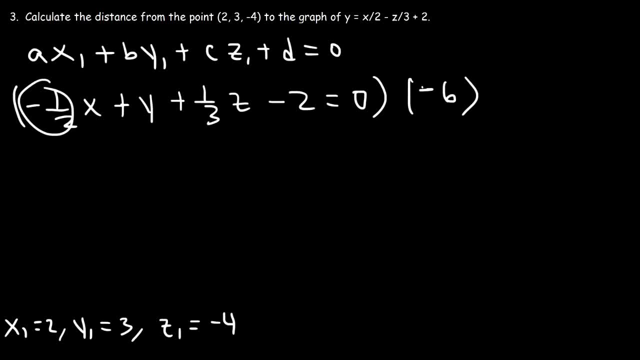 But I'm going to use negative 6 to make this positive. Negative 1 half x times negative 6, that's positive 3x. And then we have y times 3x, So that's going to be negative 6y. 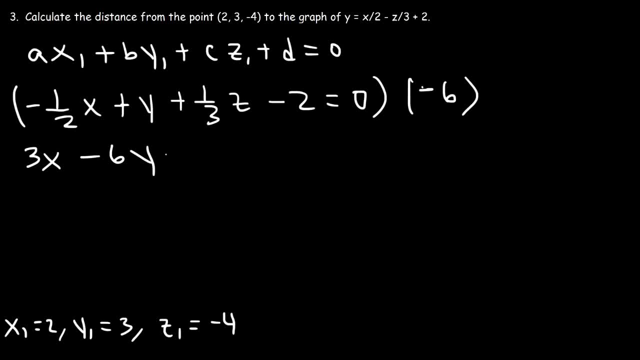 Next we have 1 third z times negative 6. So that's like negative 6 divided by 3. This is going to be negative 2z, And then negative 2 times negative 6, that's positive 12.. So now it's in this form: 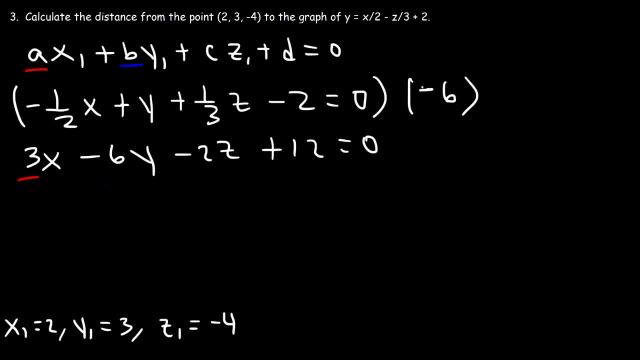 So we can see that a is equal to 3.. b is negative, 6.. c is negative 2. and d is 12.. So let's write that in the bottom. So a is 3., b is negative, 6.. 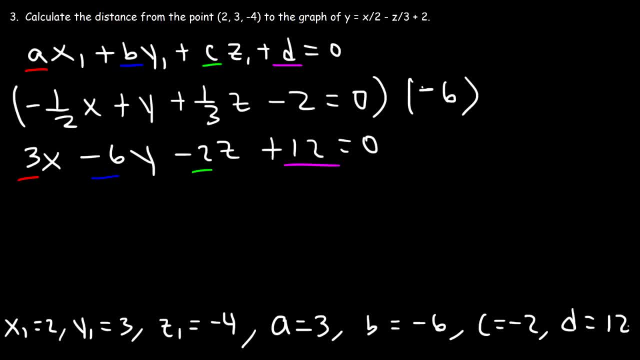 c is negative, 2. d is 12.. So now that we have all the variables, let's write the equation that we need. So the perpendicular distance between the point and the line is going to be the absolute value of ax-2. we Limit that. 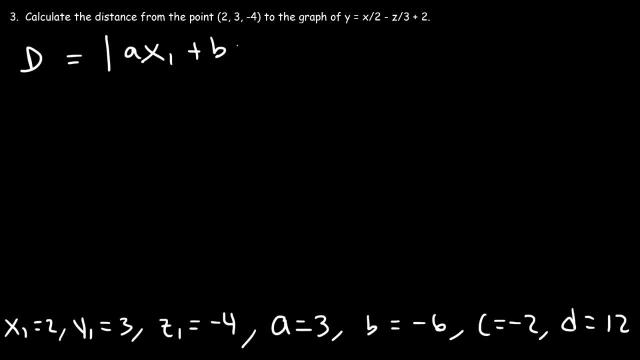 The result: QQ: X1 plus BY1 plus CZ1 plus D, all divided by the square root of A squared plus B squared plus C squared. So now let's plug in what we know: A is 3, X1 is 2..